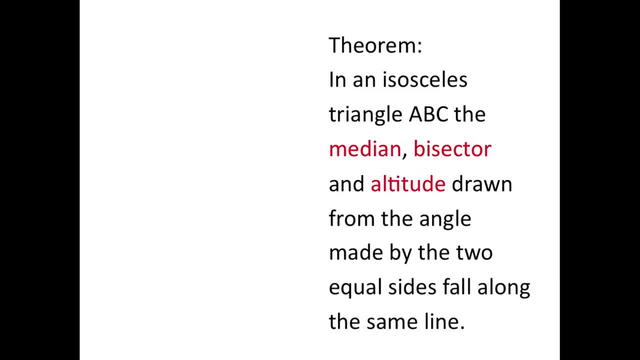 Now, to understand this theorem, we need to understand the following three terms: median, bisector and altitude. So, firstly, what's the median? Well, let's take these two triangles we have here. To find the medians of both these triangles, you have to first figure out what is the midpoint. 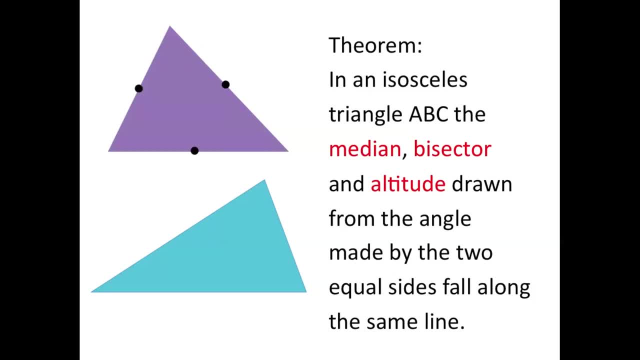 of each of the sides. So let's say, these dots represent what is the midpoint, and the median would be the line drawn from each vertex to the opposite side's midpoint. So these three lines represent the median of the purple triangle. Same way, if we find the three midpoints of the 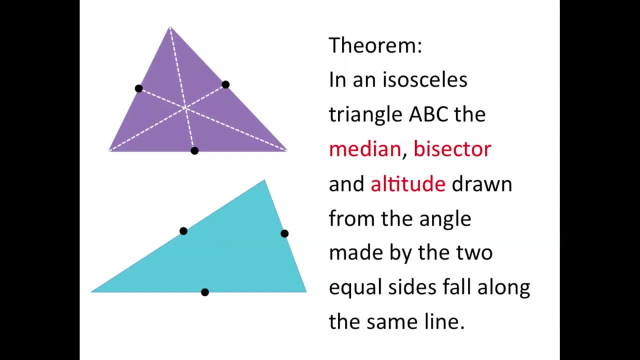 each side of the blue triangle and then draw a line from each angle to those midpoints, then we'll get the three medians of the blue triangle. Next is the bisector. So let's say that we want to find The bisector is any line drawn from each vertex that bisects the angle. 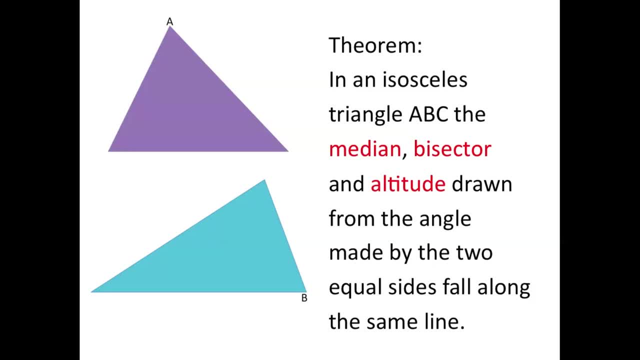 So let's say, for the purple triangle, we want to bisect angle A. then we'll draw a line from the angle to the opposite side And this one bisects the angle, which means that the two new angles created are going to be equal. 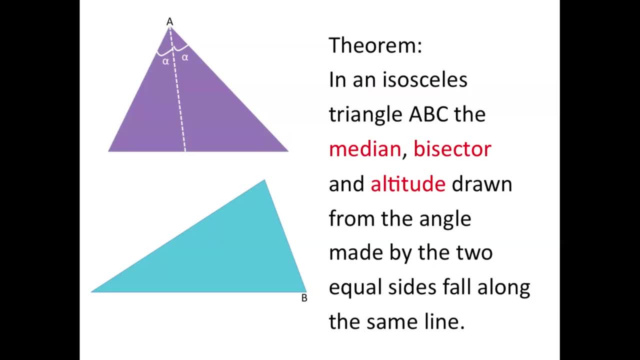 Same way, if we bisect angle B of the blue triangle, then we'll end up with two halves of angle B, which, of course, will be equal, since the bisecting line cuts the angle in half. Next is the altitude. The altitude is any line drawn from. 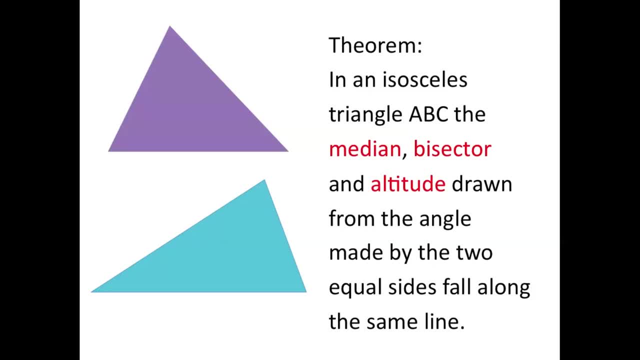 any of the vertex of the triangle straight down to the opposite side, that is perpendicular to the opposite side. So, as you can see, let's say for the purple triangle, we draw a line from the topmost vertex that is perpendicular to the opposite side, and that means that the angles created 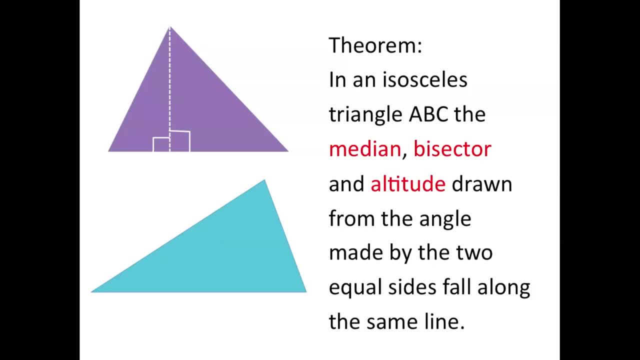 are 90 degrees or right angles. Same way. let's say, from one of the bottom vertex of the blue triangle we want to draw the altitude. We draw a perpendicular line from the bottom angle to the opposite side, which will create two right angles. 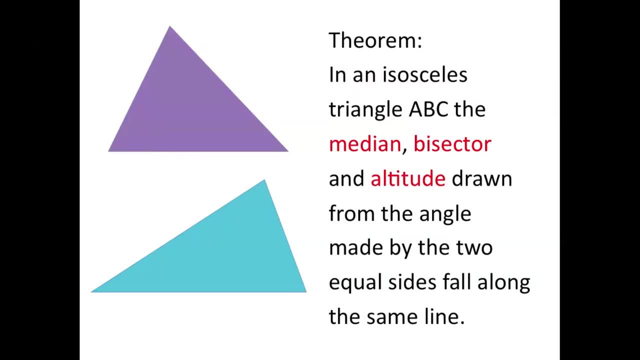 So that's what median bisecting altitude is Now, considering that we have both these triangles, if we draw the median bisecting altitude all at once on the purple triangle, we'll get this situation. So this is the median of the purple triangle. 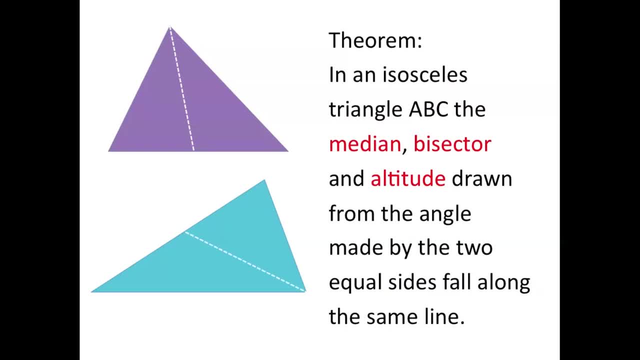 And this is the median line of the blue triangle which, if you remember, is the line from the vertex to the midpoint. Now, the bisector line of the purple triangle is this one, which basically bisects the angle that it's drawn from, or cuts it in half. 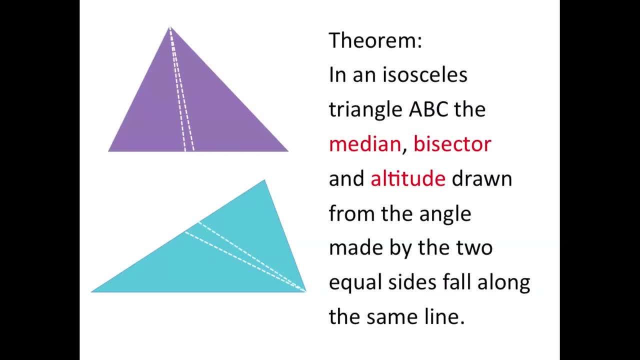 And for the blue it's this one. And next is the altitude. So the altitude of the purple triangle that we've drawn earlier was this one, and for the blue triangle it was this one. So, as you can see, all three of these lines. 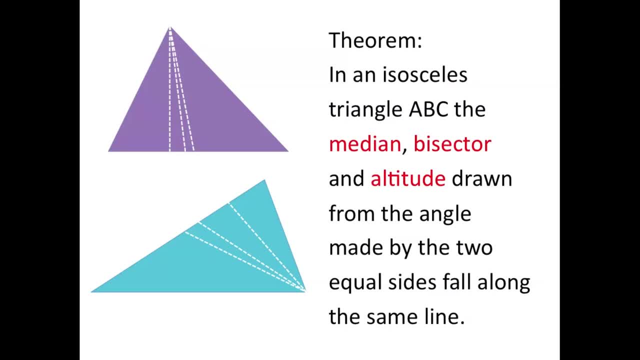 the median bisecting altitude do not fall upon each other, And the theorem is saying that for an isosceles triangle, if these three lines are drawn from the angle that is created from the equal sides, then they will fall directly on each other. 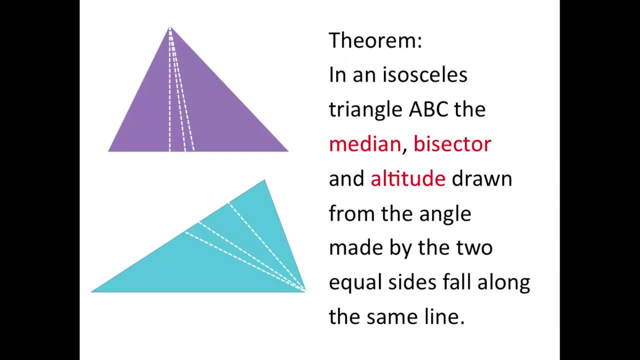 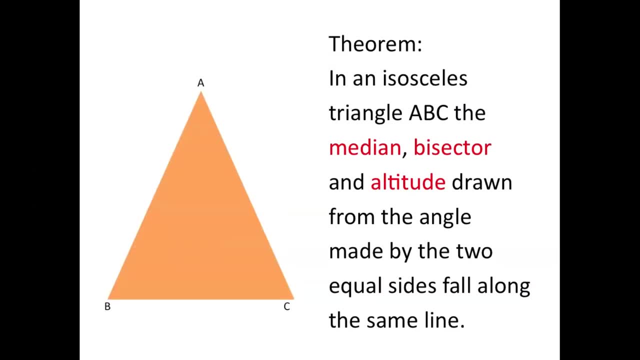 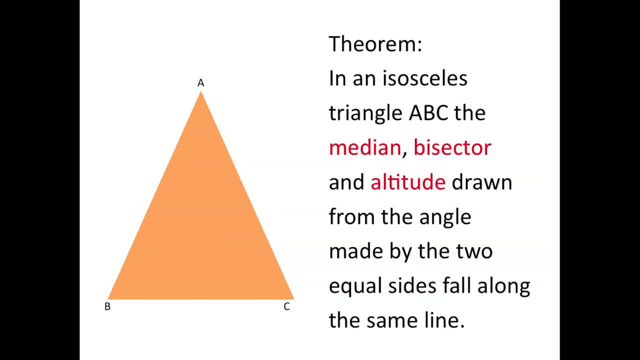 And let's say that AB is equal to AC. So that makes it an isosceles triangle, since two of the sides are equal, And we're going to try to prove that the median line, the bisector line and the altitude that are drawn from angle A are all going to fall on the same line. 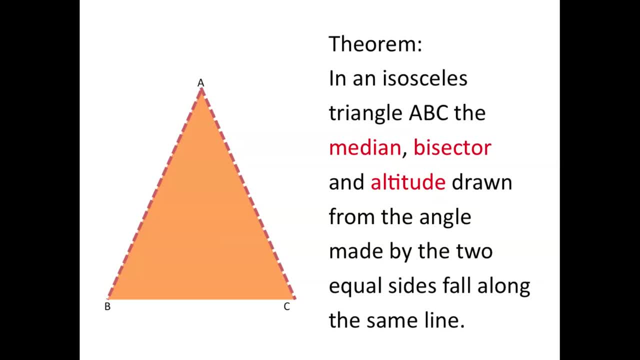 So to show this, the first thing we're going to do is draw the median of our isosceles triangle, ABC, So median. to draw the median we have to first denote what's the midpoint. So let's say D is the midpoint of side BC and we're going to draw the median line from. 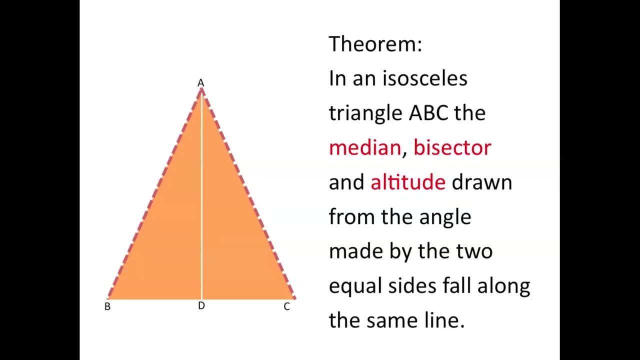 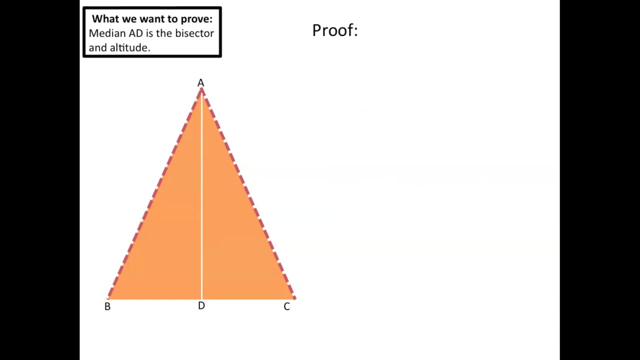 A to D And now that we know this is the median, we want to also prove that this is also the bisector and the altitude of this triangle, And I'll show that the theorem holds true. So, beginning with our proof, we already know that AB and AC are equal and since we said 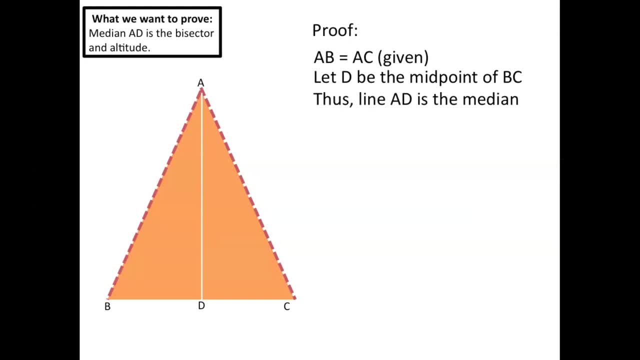 earlier, we're going to make D our midpoint of BC, which makes AD the median. So, keeping all this in mind, we know that BD has to be equal to CD, because we've already said that D is our midpoint. Also, we know that angle ABC has to be equal to angle AC and we know 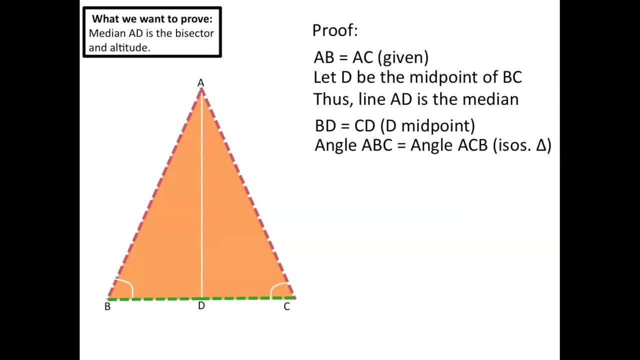 ADB because ABC is a, a self-laze triangle. So now with that information we can al- we can now say that by side angle, side ATR is congruent to UACD because side AB and AC are equal, side B and CD are equal and the angles B and CD are equal aresehen every. 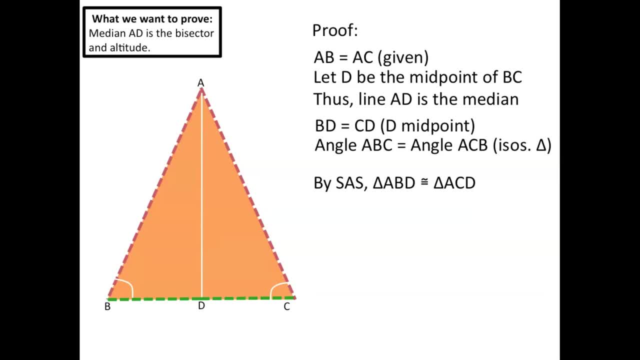 side is congruent, 3 between them is also equal, proving that these two triangles are congruent. So because they're congruent, we cannot say that the angle BAD is equal to the angle CAD, And if those two are equal, then that means that the line AD has bisected. 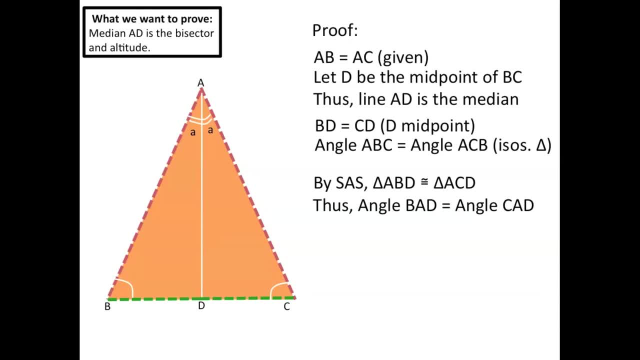 angle BAC. So that makes AD the bisecting line of angle A. So now we've proven that AD is bisecting line and all that's left to do is to prove that AD is also the altitude. Well, as you can see, because we said earlier that triangle ABD. 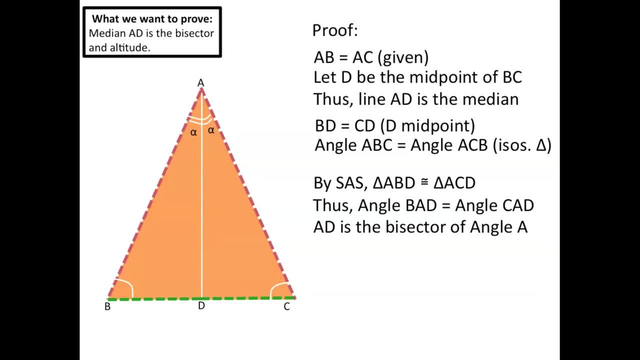 is congruent to triangle ACD. we know that angle ADB, which is right here, it has to be equal to angle ADC, which is right here. And also this line, BDC, is a straight line, so it's 180 degrees. So the only way this angle and this angle can also be, can be equal and 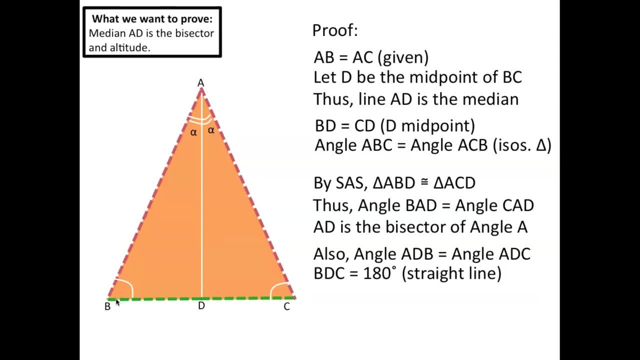 also result to a 180 degree straight line is if they're both 90 degrees. So since we have two 90 degrees degrees here, then that proves that line AD is the altitude of ABC. Thus that shows that in an isosceles triangle the median, the bisector and altitude lie on. the same line.